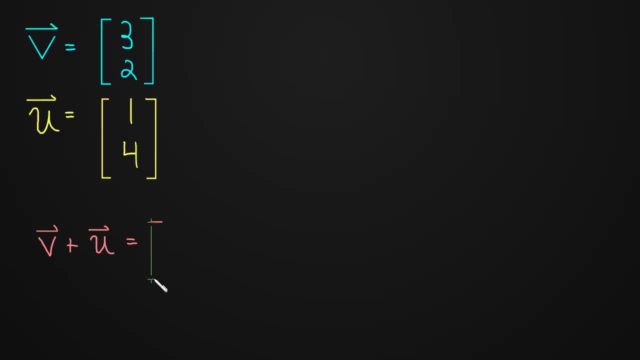 So u plus v or v plus u- I should say v plus u- is simply going to be. we're going to take the two vectors and add them. so I'm running out every step here. And how do we do this? 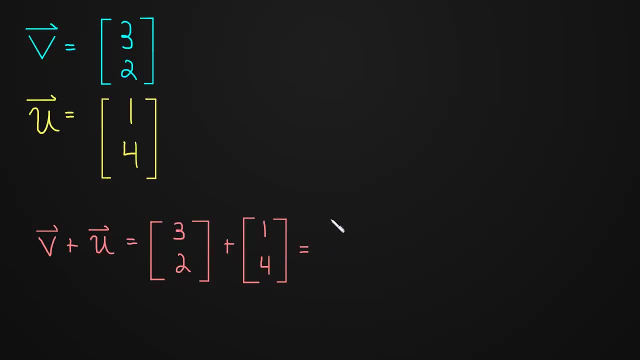 Well, we just add their corresponding components together. So the first component of v plus u is just going to be the first component of v, which is 3, plus the first component of u, And you can see just visually. you can see what's happening here. 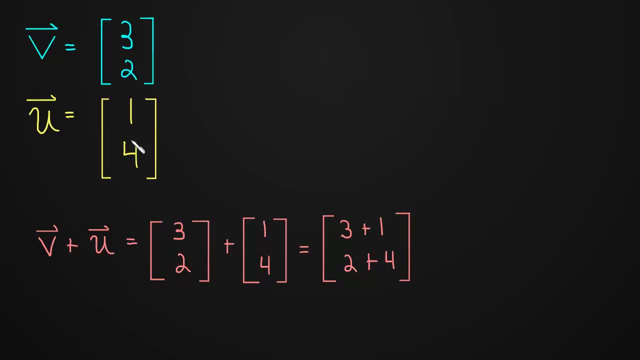 The second component of v plus u is just the second component of v plus the second component of u, which in our case just becomes 4, 6.. So when we add vectors together we get a new vector, And here we got the vector 4, 6.. 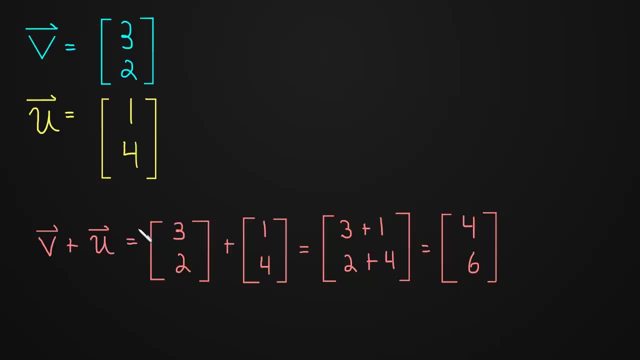 Okay, so just to save some space, let me erase these steps here. I'll move this over. Okay so let's now look at this on a graph. Here is u and v: U in yellow, v in blue. Real quick, because I haven't mentioned this yet. 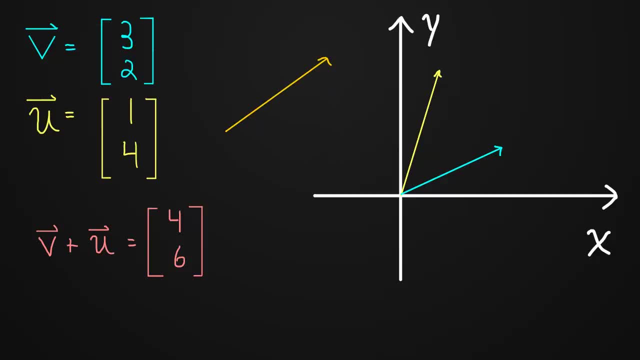 vectors have two things. One is called a tail, its starting point, and the other is called a head, its ending point. I mean, they have more than two things, I guess, but they have a head and a tail. So when we add vectors we line up their tails at a common point. 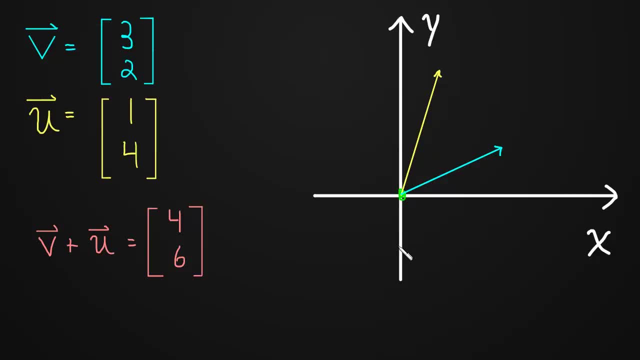 Here we pick the origin just because it's convenient. So we line up their tails at that common point And then to add them we just take we're going along- v, and then we take u and place its tail to the head of v.